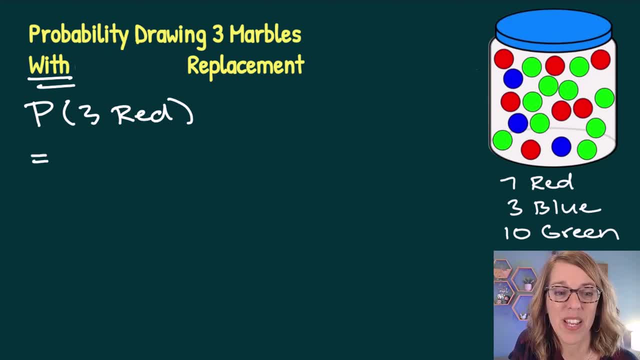 the second marble, The probability of three red becomes the probability of getting the first one red and the second one red and the third one red. I can also rewrite this using that and instead as a multiplication. So I want the probability of red times the probability of 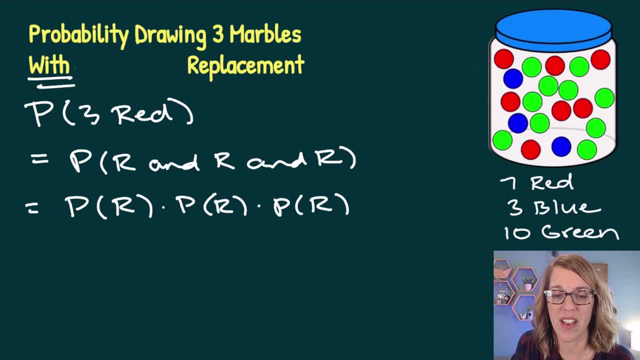 red for the second draw times: the probability of red. Well, as I go in to draw that first red marble, I know that there are seven of them out of the total seven plus three marbles. So I'm going to go in, and I'm going to go in, and I'm going to go in, and I'm 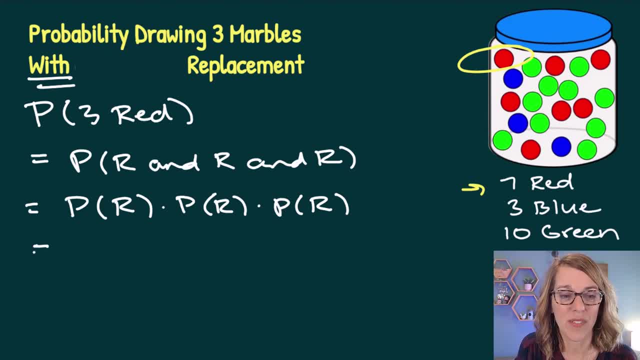 going to say three plus 10 is 20.. So when I do that first marbles probability, I assume it's red and there are seven favorable out of 20 total. Now I go in to draw the second one, I'm putting that first marble back in. So when I go to draw the second red, I'm assuming it's red. There are 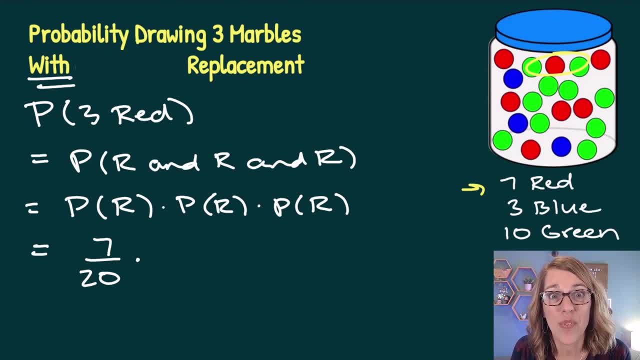 still seven of those red marbles out of the 20 total marbles in the jar. So I have another seven out of 20.. I draw that red marble, put it back in and I end up with again: there's seven red marbles. 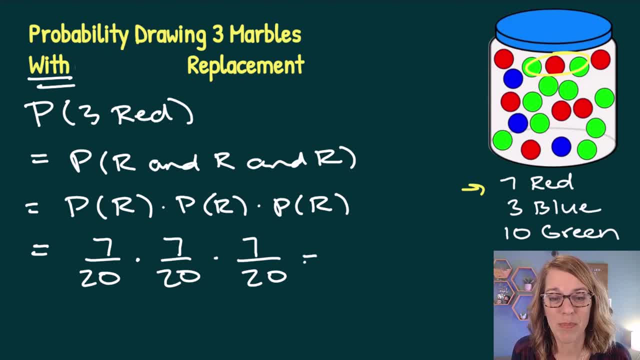 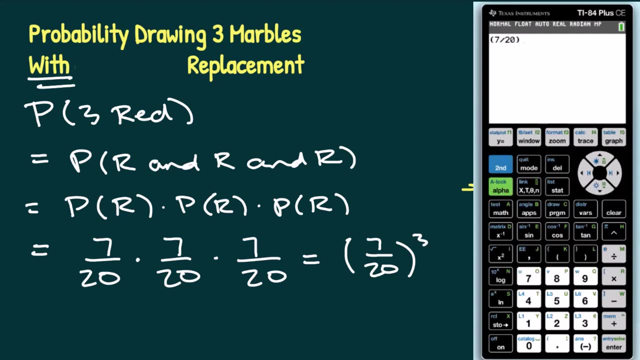 out of the 20 total. I can go ahead and multiply these three together. I can also write it as seven twentieths to the third power. Let's put this into the calculator. So I'm going to go- parenthesis: seven divided by 20.. And let's do this to the third power. So caret three enter, I end up with. 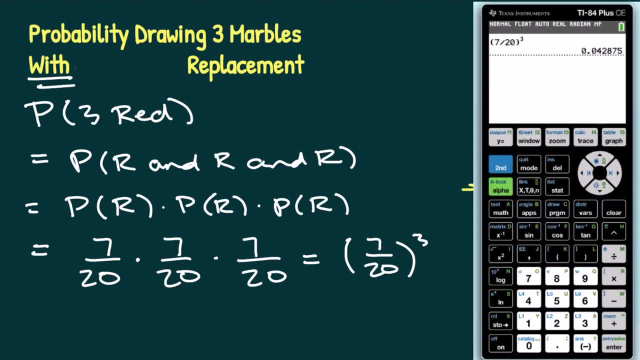 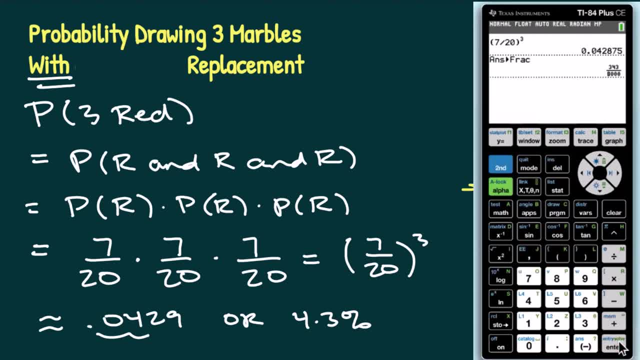 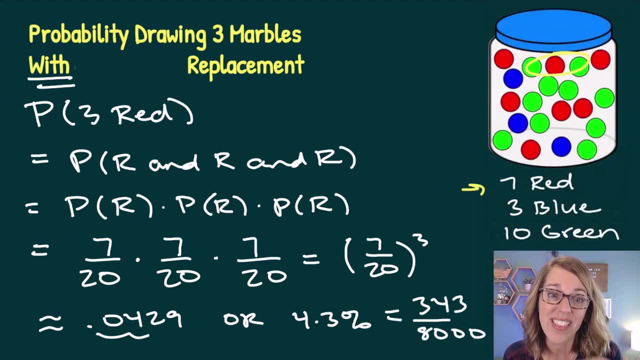 oh, you want your answer as a fraction, and I do, and I hit enter and it gives me that 343 out of 8,000.. So I can also write this as 343 out of 8,000.. Okay, now, let's do this without. 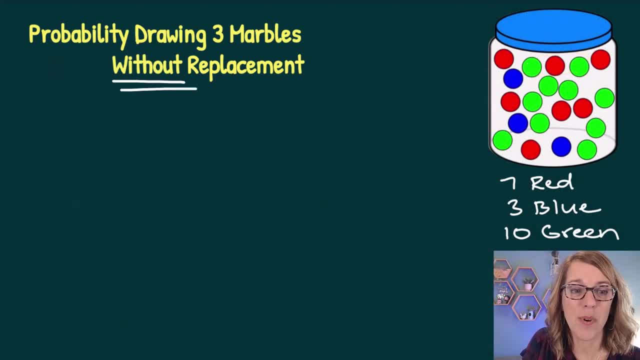 replacement. I've got that same scenario, but without replacement. when I go and choose each red marble, I'm going to choose a marble and once I've drawn it out of the jar it's gone and I'm going to go back in with one less marble, but my probability ends up being the same setup. 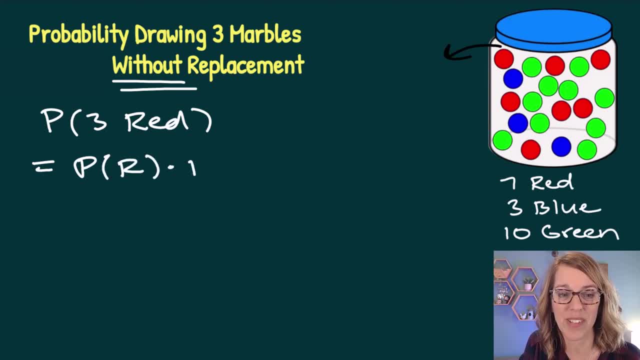 So I'm going to have the probability of a red and which is going to be multiplied the probability of red, and so I'm multiplying that probability of a red. Now let's go in and draw that very first marble. I'm going to go in and draw that very first marble and I'm going to 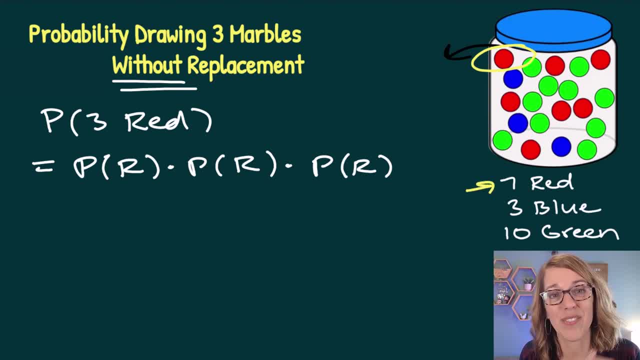 assume that it's red. There are 7 out of the 20 marbles total. so when I draw that very first marble, I end up with a probability of 7 out of 20.. Now here's the difference: I've drawn that. 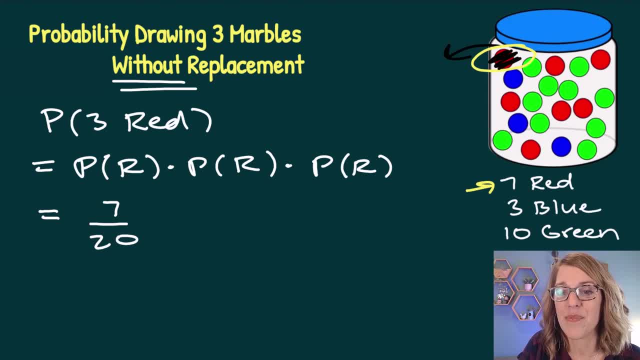 first red marble and I'm going to now get rid of it, which means that instead of 7 marbles, I now have 6.. 3,, 4,, 5,, 6.. So I now have 6 marbles remaining. 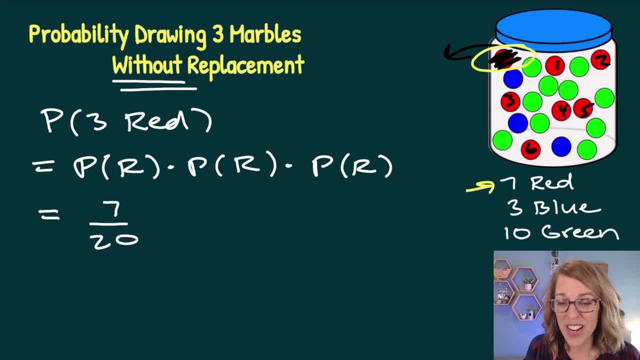 And instead of 20 marbles total, I've taken one out, so that means that we have instead 19 marbles. So when I go to do the second probability, I've taken one red marble out, So there are 6 red. 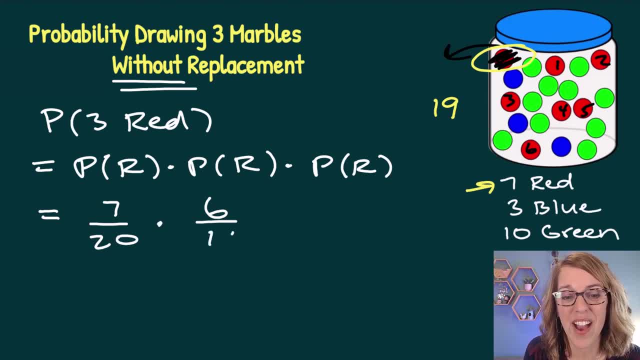 marbles out of. since I took a marble out out of the 19., Let's go ahead and take another red marble out. That means that I've got 19 marbles. So I've taken one red marble out and I've taken 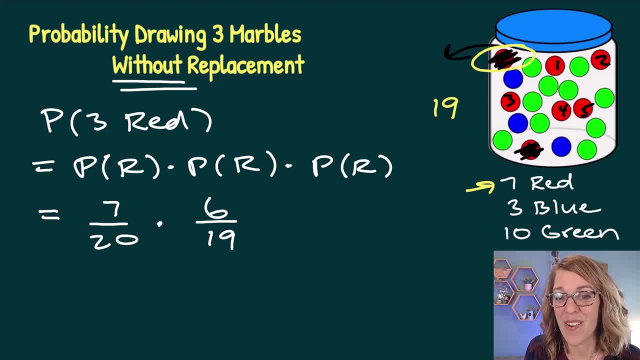 now 5 red marbles left, and I've also reduced the total number of marbles to be 18, because now I've drawn 2 of those out And notice how, as we're doing the probability I assume that they're a red.